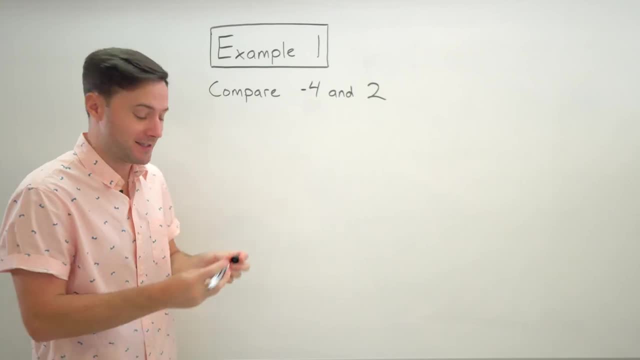 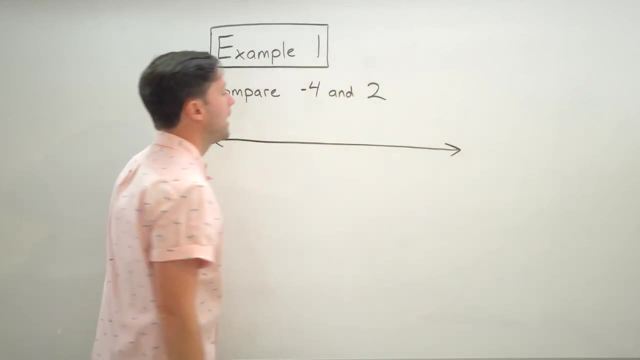 so naturally, you probably guessed, I'm going to use a number line to help me figure this out. So I'm just going to start with my arrows at both ends, which is really important. And now, normally, if you're not super comfortable with drawing number lines, you might want to put: 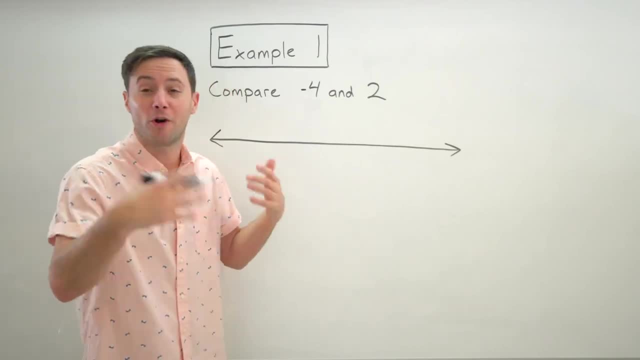 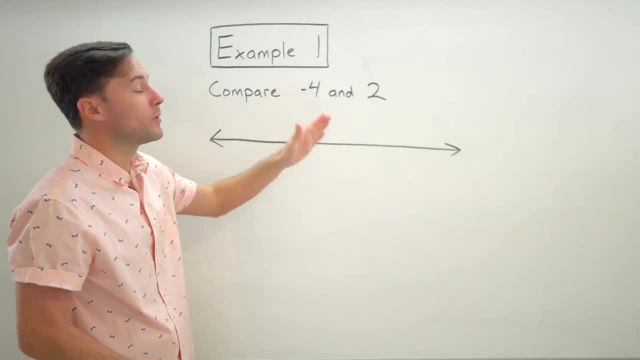 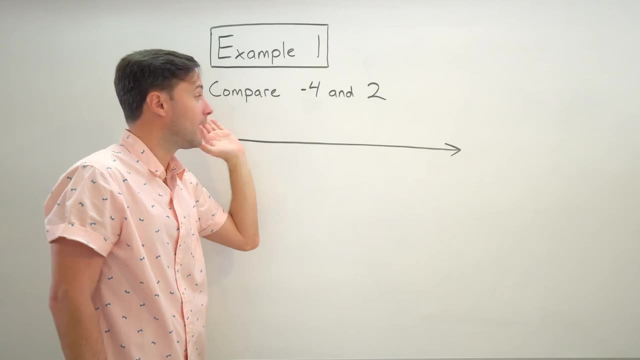 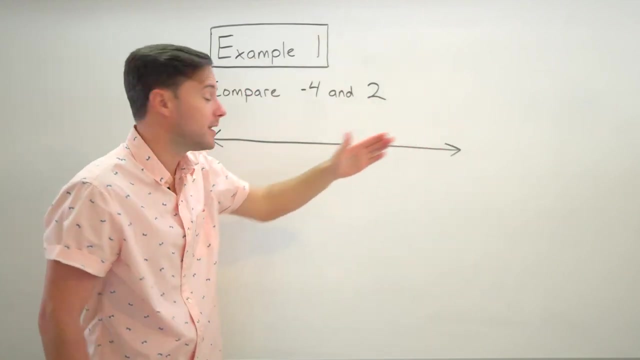 could pick one of these values, So for me I'm going to start with negative four. I know negative four is going to be left of negative two on the number line because it's negative right. The negative integers are to the left of zero. Positive are to the right. So I'm going to start. 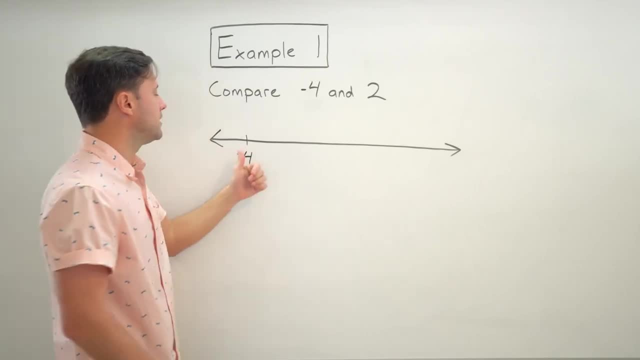 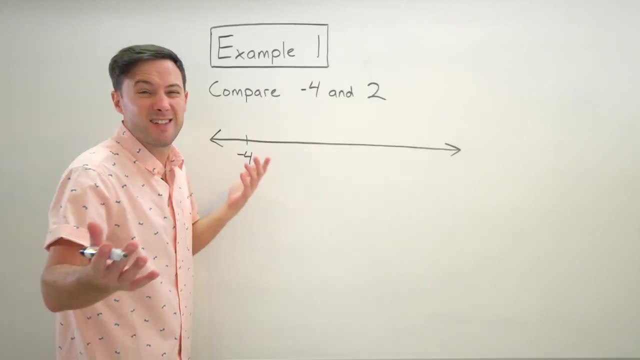 with negative four down here. I don't need to go any less than that because I don't need to compare a number less than negative four, And then I'm just going to. I'm going to because I only have to go to two. I'm just going to count by ones, making sure that my spacing is consistent. So that would. 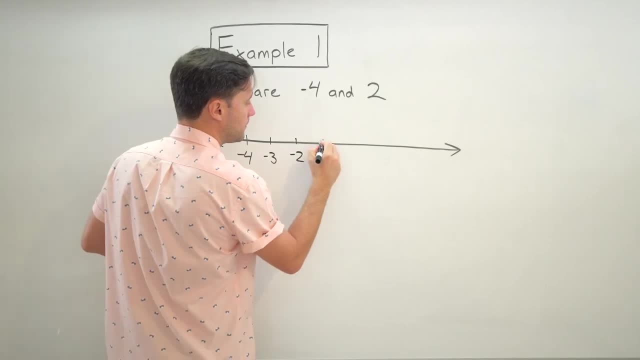 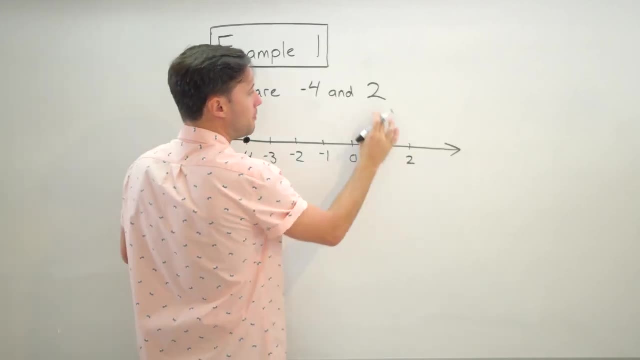 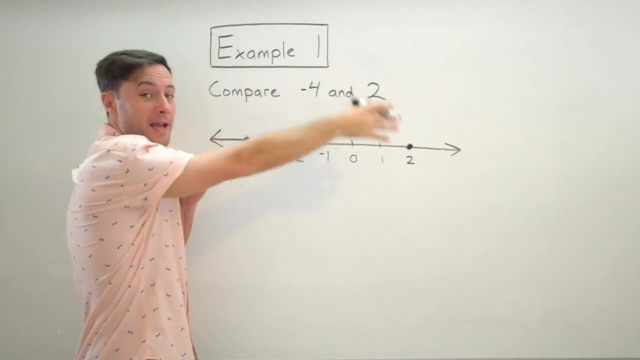 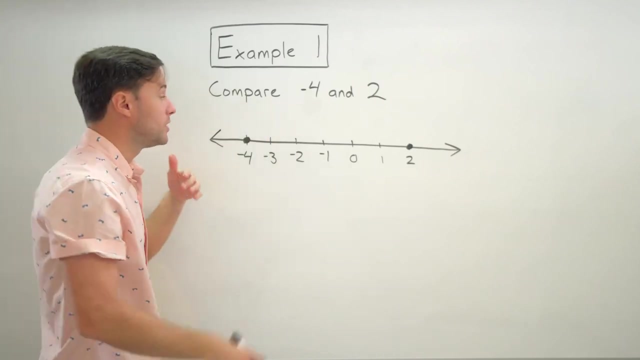 be negative three, negative two, and that would be two. So negative four would be here and positive two would be here. Well, we know that as you move to the right on the number line, the values increase, And as you move to the left, the values decrease, which means 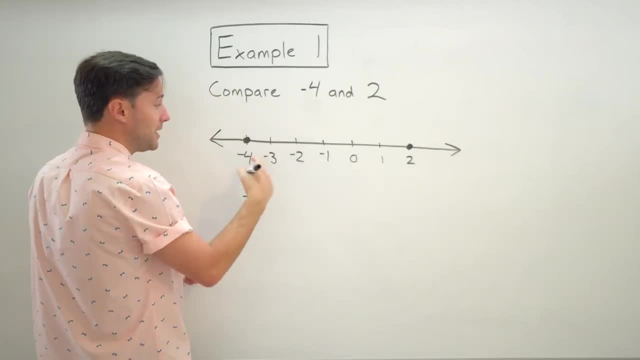 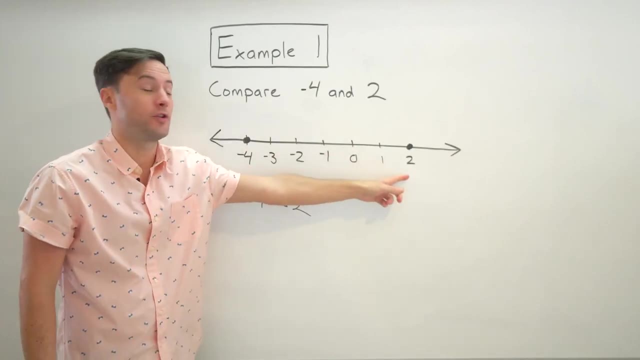 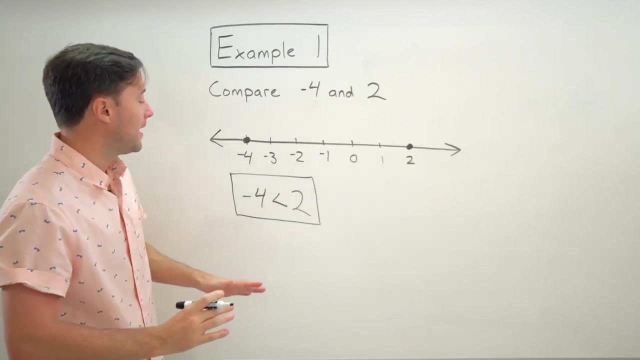 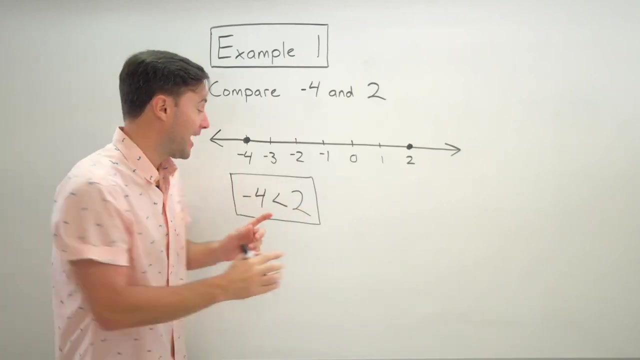 negative four has to be less than two because it's to the left of two on the number line. Okay, Now I know a lot of people kind of get in the habit of just thinking this is maybe just one symbol and you just switch the numbers around. No, no, no, There are two symbols. There's a. 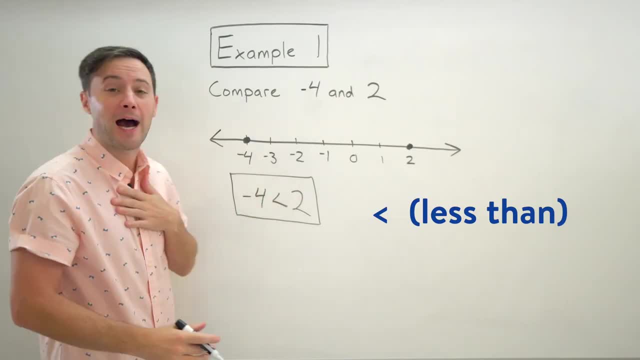 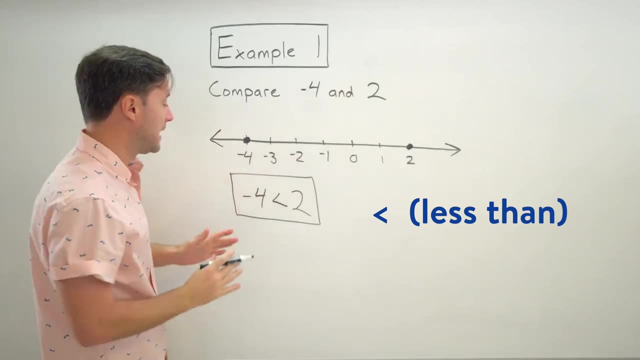 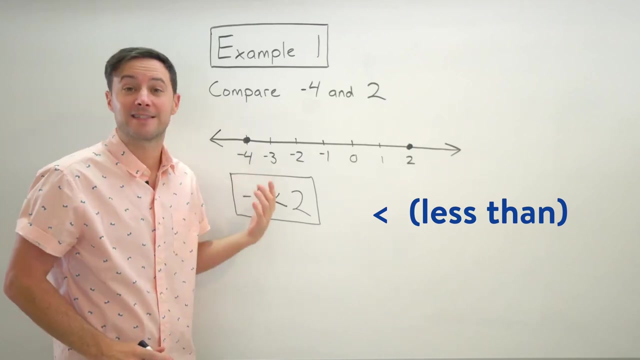 less than symbol. that looks like this, And I always think about it. We read left to right. right, When we read a sentence, we read left to right. If you're reading English, I should say So. I just remember it as left to right. If the small end is first, that's less than, And then 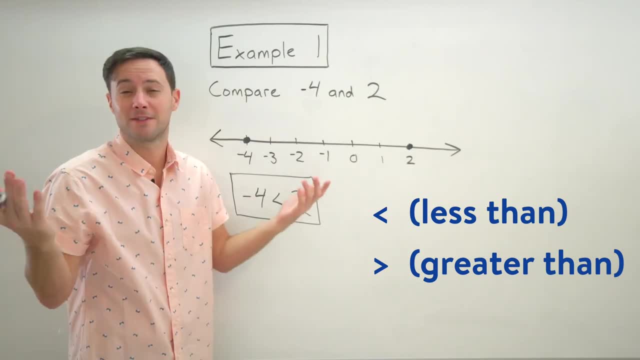 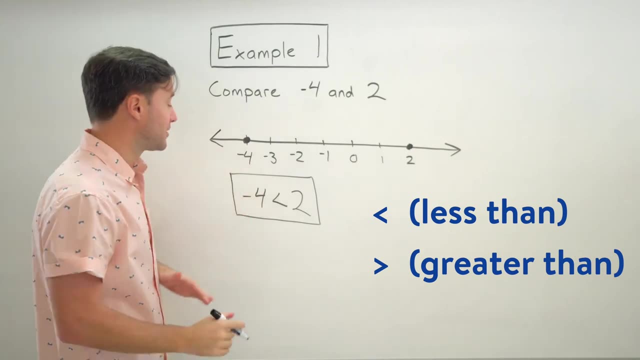 the other one left to right. you see the big end. Some people think it's like the alligator open his mouth. That is greater than So. there's actually two different symbols. Just making sure everybody understands that. All right, let's try another example. Okay, we're comparing two numbers again. 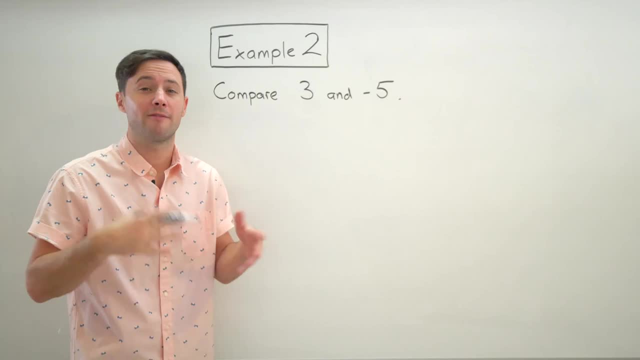 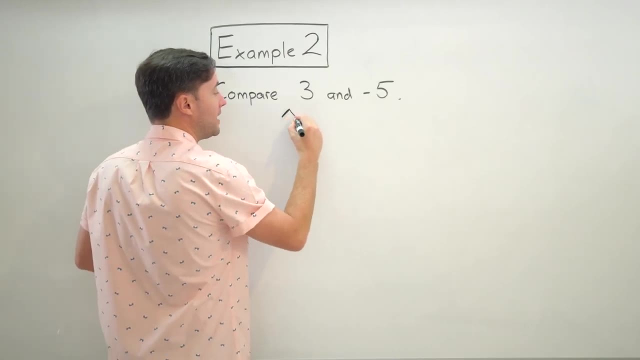 but this time I'm going to draw a vertical number line just to show you kind of how that looks a little bit different. So we're comparing three and negative five. Same thing. We need arrows again, but this time I'm drawing it vertical, which really doesn't change much. So I'm going to draw 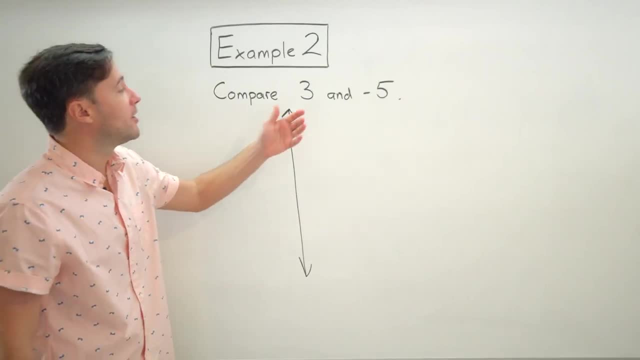 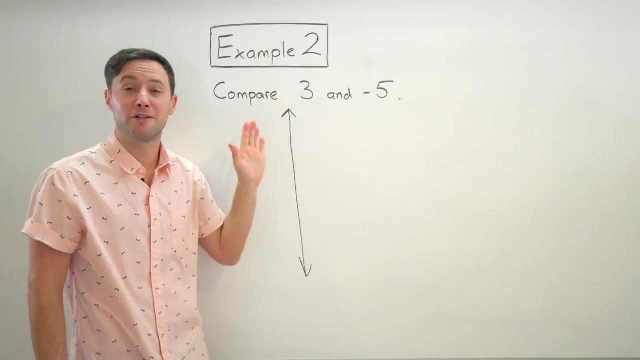 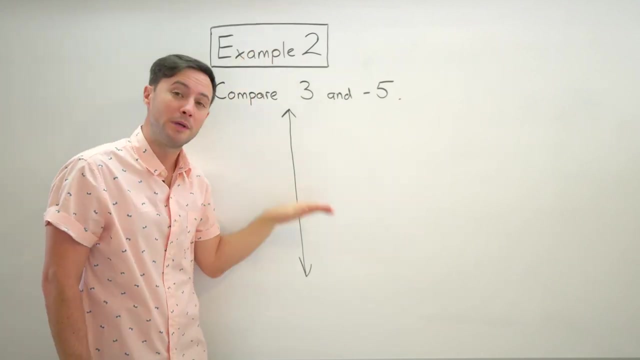 my vertical number line. I'm going to say: I know three is positive. Now the positive integers are going to be above, instead of positive integers to the right of zero. Now we have a vertical number line. Positive integers are above zero, Negative would be below. All right, so I'm going to start. 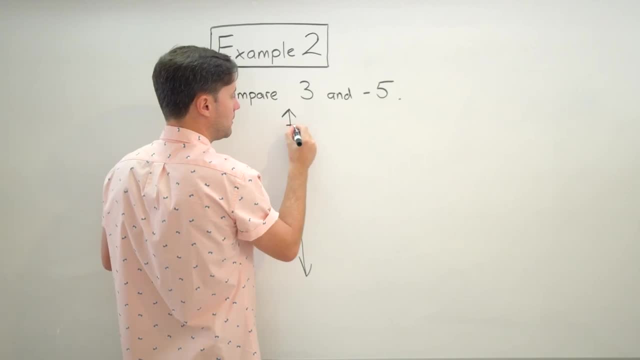 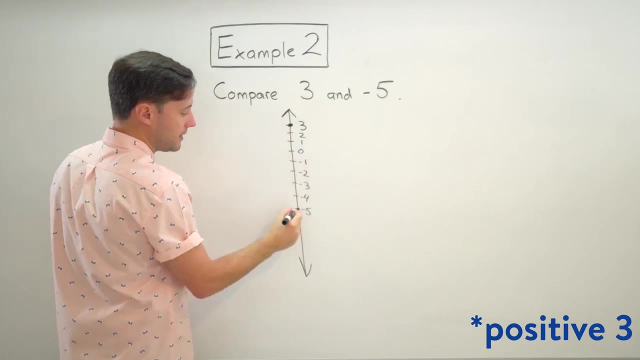 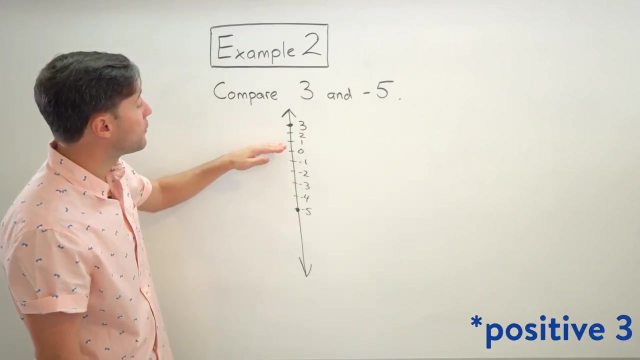 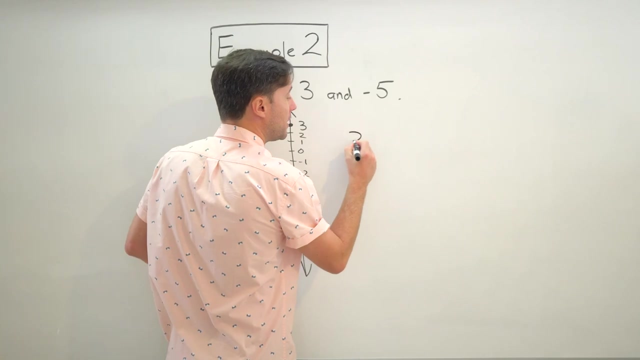 with three all the way at the top of my number line. So there is three. So here is negative three and here is negative five. So again, how can this help us compare them? Well, negative three is above negative 5 on the number line, which means 3 is greater than negative. 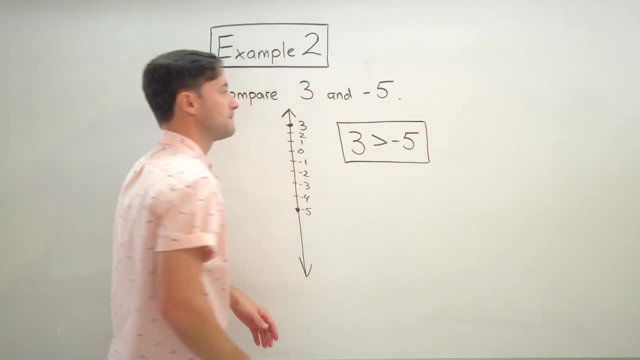 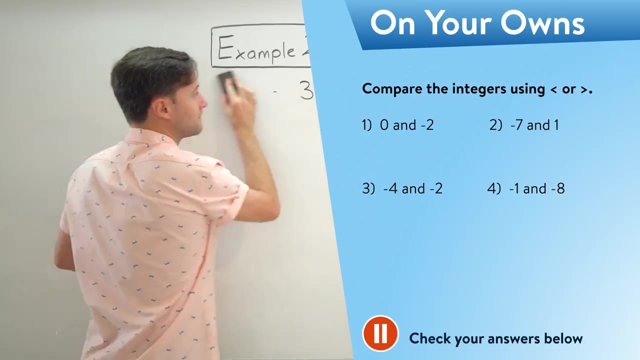 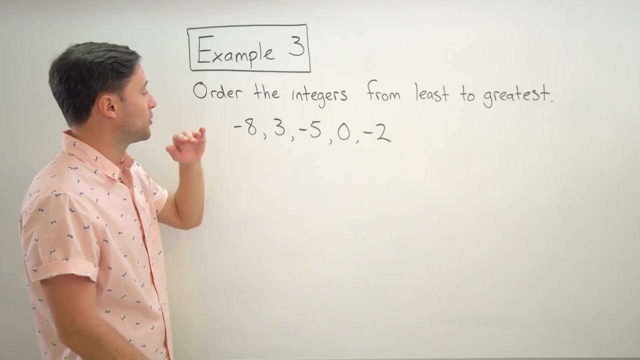 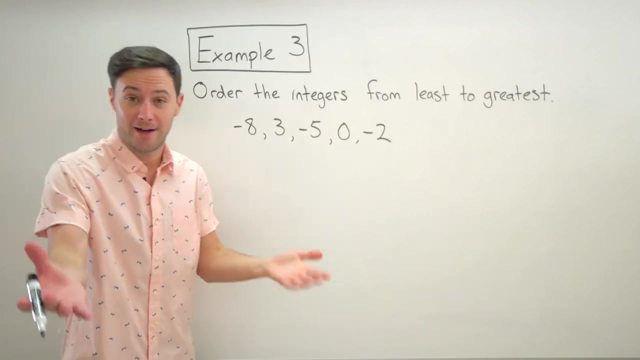 5. all right, hopefully that helps. here are some to try on your own. all right, here's our last example. order the integers from least to greatest. so here are our integers. we've got some negatives, we got one positive, I guess, and we've got 0. so again, I'm going to use a number line to help me, kind of. 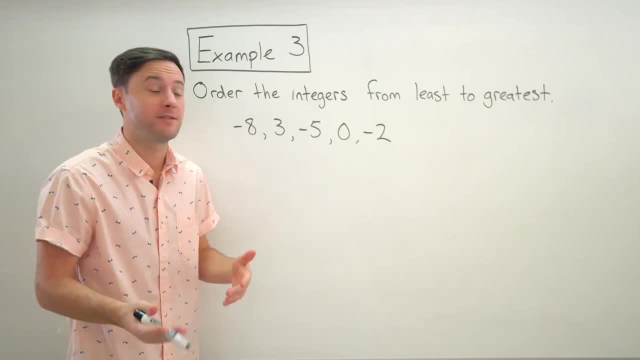 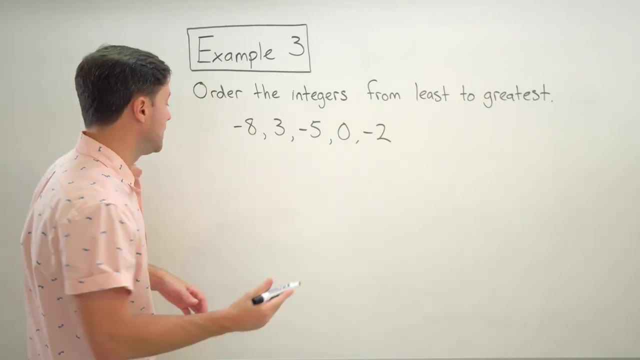 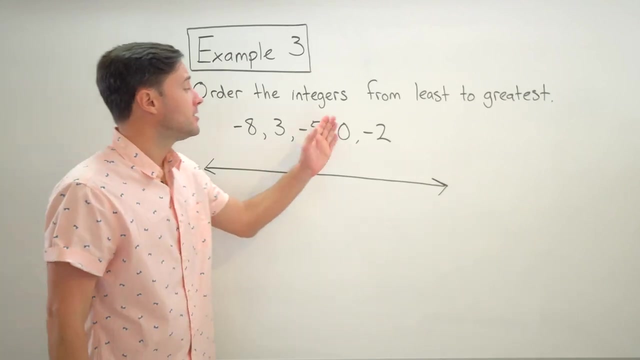 figure this out as you get more kind of comfortable with this. you might not even need and a number line to help you order these from least to greatest, but for right now we're going to make one. so again, here we go. we've got my arrows like that now. just because there's zero doesn't mean I have to put. 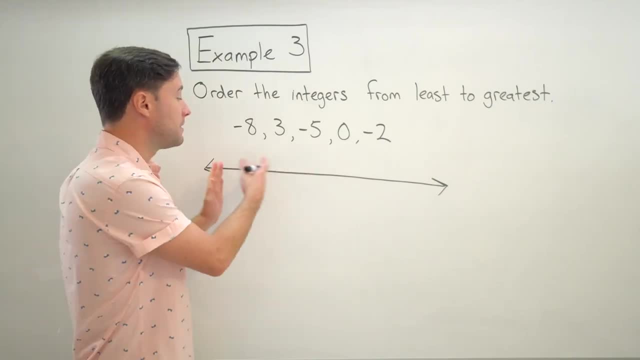 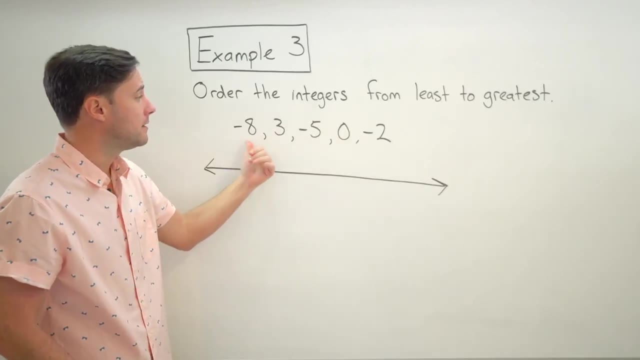 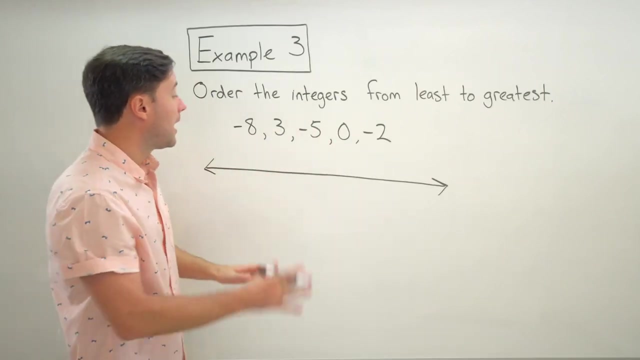 zero right in the middle. That might kind of limit me with space. If I look I know I have to go all the way down to. it looks like negative eight would be my least and it looks like three is my greatest. So I probably need more space on the negative side. So when